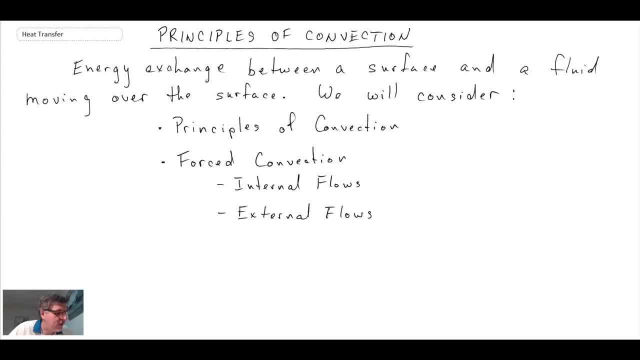 External would be an example of the flow within a pipe. External flow would be the flow over a heated fin, for example, where you're forcing the fluid to go over that fin. We'll also be looking at free convection, sometimes also called natural convection. 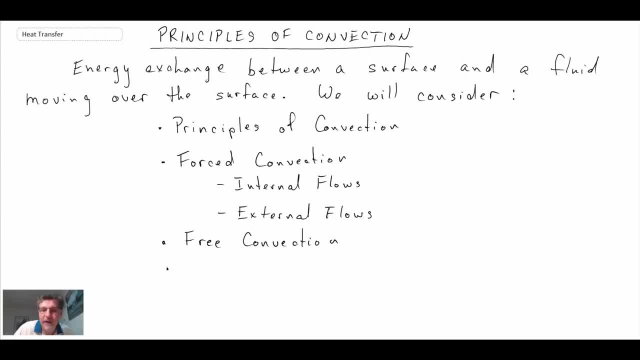 And we'll be looking at convection with phase change, And we refer to this. there are two types that we'll be looking at: boiling and condensation. And finally, we'll be looking at convective heat transfer when we study heat exchange. 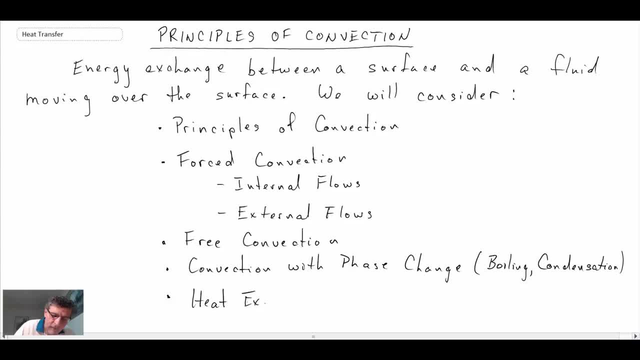 There's an Obama-Bennett law which says that the temperature changes through heat transfer, and you're going to be looking at convection instead of the temperatures. So you can see, we're going to be looking at convection quite extensively for the remainder of the course. 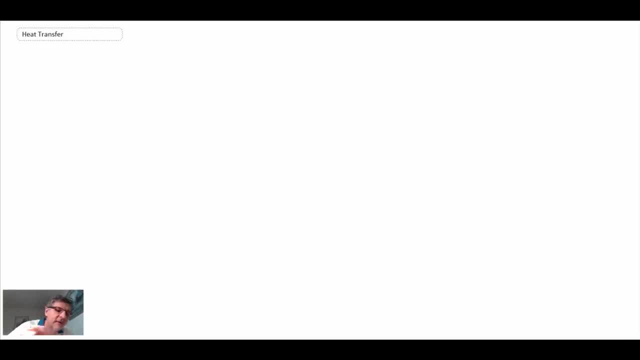 And, if you recall, the equation that enables us to quantify the amount of convective heat transfer was Newton's Law of Cooling, Convection, Equality, Cooling. Cooling Convection, Equality, Convection, Equality. law of cooling. we have a temperature differential between our free stream velocity and the wall. 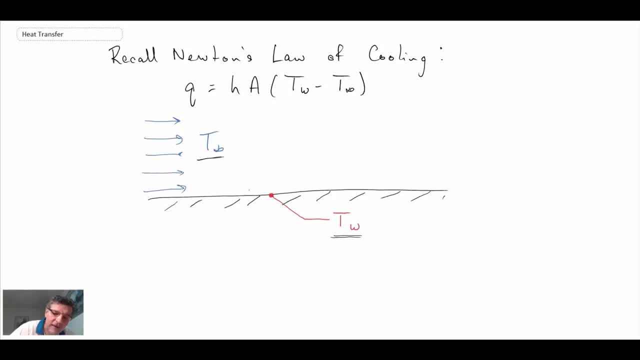 temperature, and the net consequence of that is that temperature differential results in energy exchange or heat transfer, either from the wall to the fluid or from the fluid to the wall, dependent upon which is larger, and so we've been using this over and over and over again throughout the course. 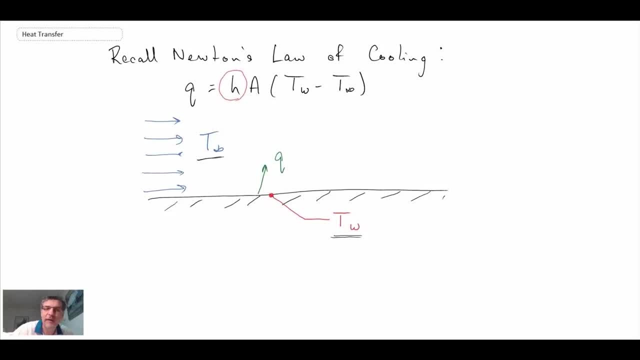 but one thing that we haven't really addressed is: where does h come from? and so that's what we're now going to set out to determine is how to quantify h. okay, so in determining h, there are a couple of different ways that we can do this. 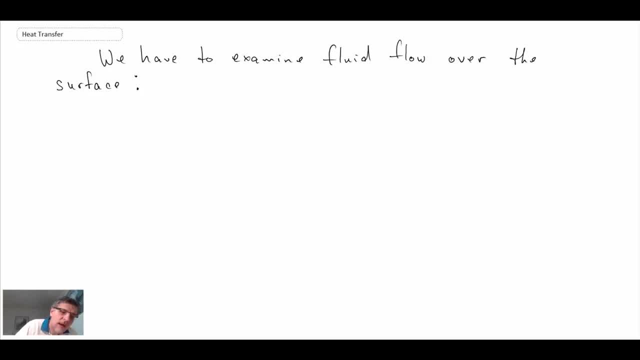 now, given that convective heat transfer involves a couple of different ways that we can do this, fluid flowing over the surface. we need to examine that fluid flow in order to be able to quantify the value of h and, consequently, what we're going to be doing, we're going to be looking at. 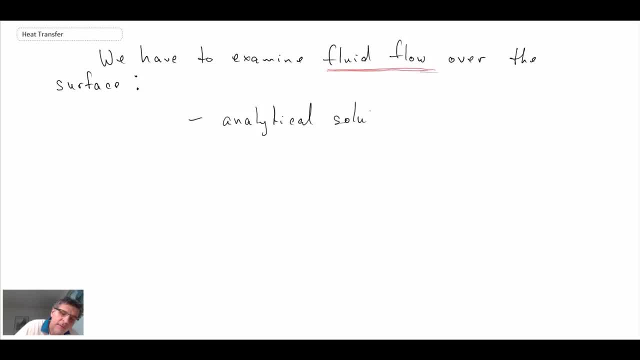 analytical solutions, and there are only a limited number that exist, and the reason for that is: if the flow is turbulent, we have no analytical solutions for the particular fluid flow flow field, and otherwise it's only for fairly restrictive geometries that we can get an analytical velocity profile, from which we could then get the temperature profile using the energy. 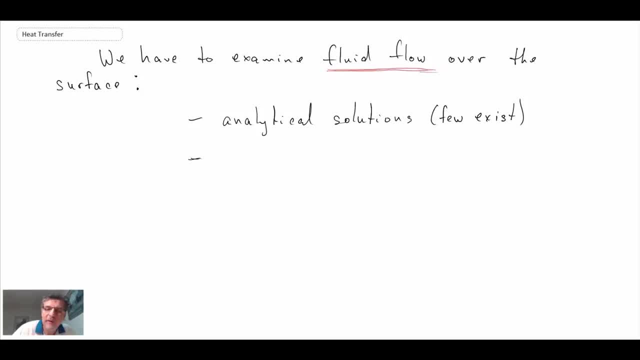 equation, and so we'll use analytical solutions. we'll look at a few, and but for the most part, what we do in heat transfer- convective heat transfer- is we use empirical data, and and so this is data that we're going to be using, and we're going to be using data that we're going to be using. 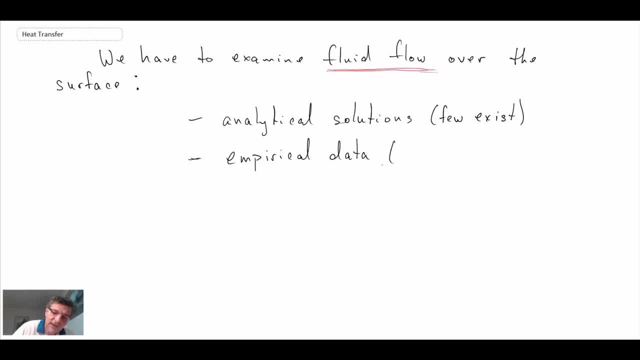 that has been collected via experimentation and this is quite widely used, and so what you're going to find is we're going to be using different values, mainly the connective heat transfer coefficient, that will be embedded within non-dimensional numbers, and and that data has been collected experimentally and then collapsed into these non-dimensional numbers to give it. 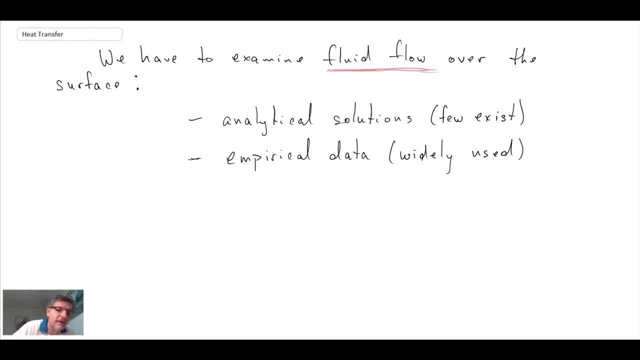 application to geometries that are different from the ones that are studied in an experiment. so they would scale geometrically, but but they they would be either subscale models or things like that. so, anyways, we'll be looking at that as we look at convective heat transfer. so it really what that means is that convective heat transfer within the 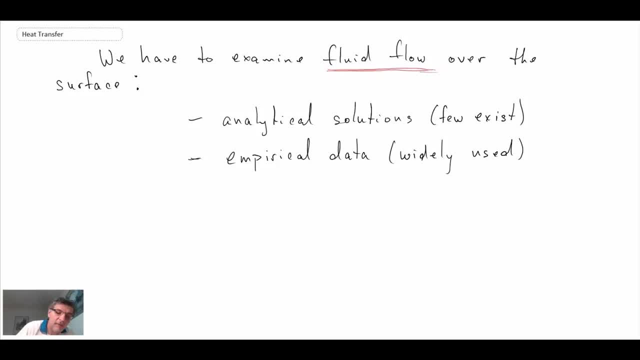 heart of it. it really is a fluid mechanics problem, and the other thing that we'll find is the convective heat transfer coefficient. we'll find that the convective heat transfer coefficient itself will often come from experimental data and, like I said, it will be represented in non-dimensional numbers for force. 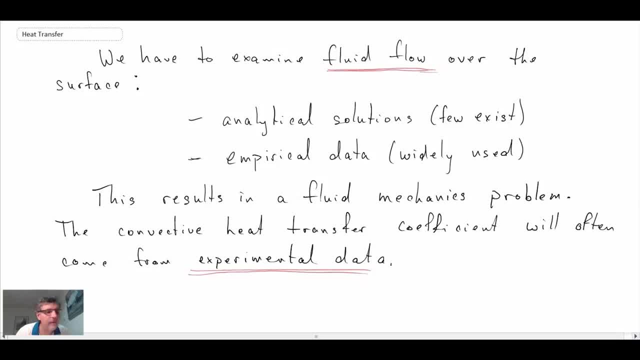 convection. quite often we're using the new salt number, which is a number that we'll be taking a look at, but that's what we're going to be doing. so we'll be doing a lot of fluid mechanics in this lecture and in the next couple, and and then it turns into a matter of collapsing.